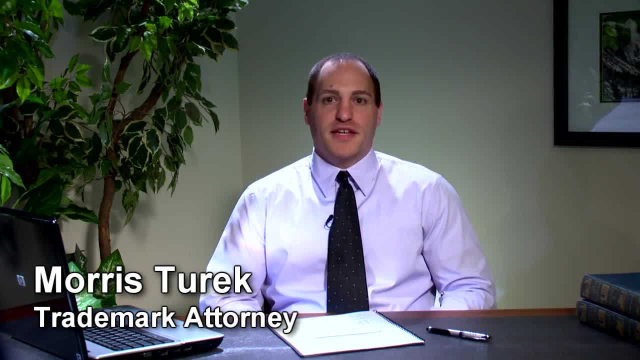 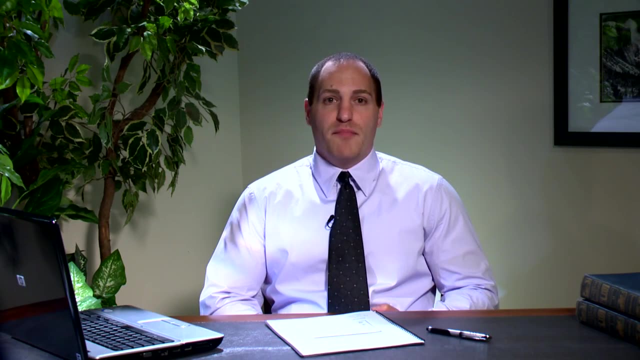 Hi, I'm trademark attorney Morris Turek. I protect individuals and businesses throughout the world by assisting them with their important trademark matters. If you're, like most people, in need of trademark services, you are concerned about cost, and rightfully so. You have a budget and need to. 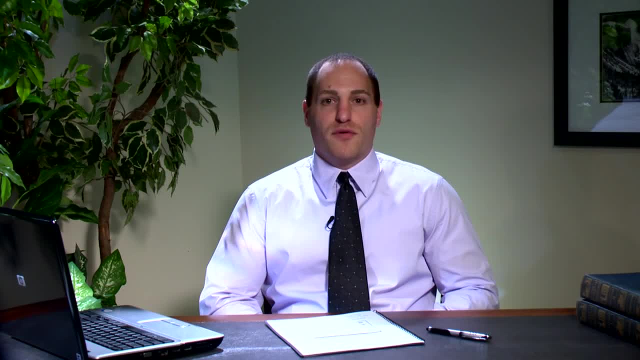 stick within that budget so that you can afford all of the other important things you need. But when you're looking for someone to help you with your trademark search or trademark application, it can be tough to figure out where you can get the best value for your hard-earned dollar. 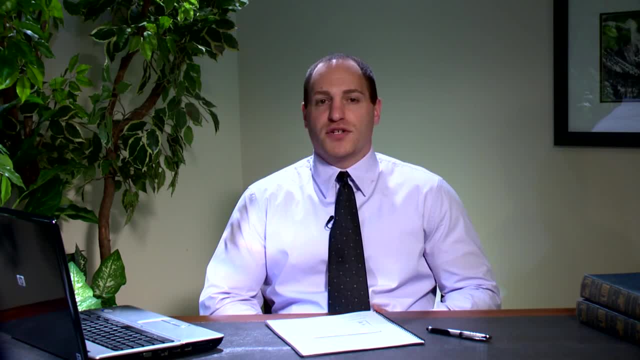 Unfortunately, a lot of people will use a document preparation service like LegalZoom. Because LegalZoom is not a law firm and cannot offer you legal advice or guidance. it is no wonder that LegalZoom's services are extraordinarily inexpensive. But cheap does not equal good value. Without legal advice, how will you know if it's in? 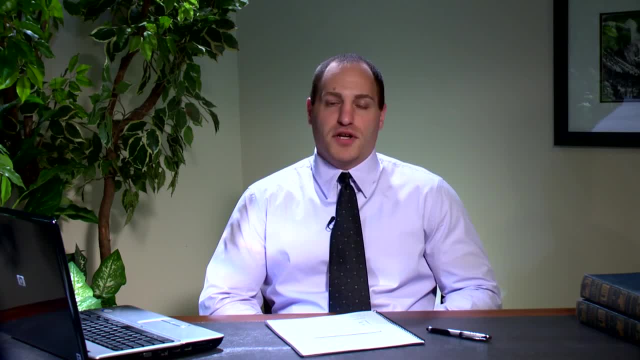 your pocket or not. If you're looking for someone to help you with your trademark search or trademark application, you will need to find someone who is in your best interest to adopt and attempt to register a particular trademark. How will you know that you won't be sued for trademark infringement? 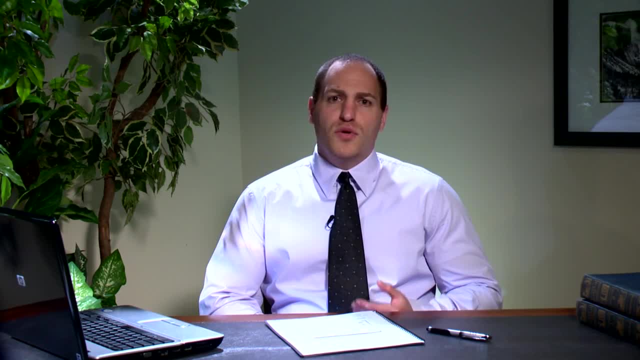 The simple answer is that you won't. You can also find trademark attorneys all over the United States who will perform your trademark search and prepare your trademark application at a highly discounted rate. Many of these trademark lawyers will boast about how cheap they are compared to their competitors, But you have to ask yourself whether 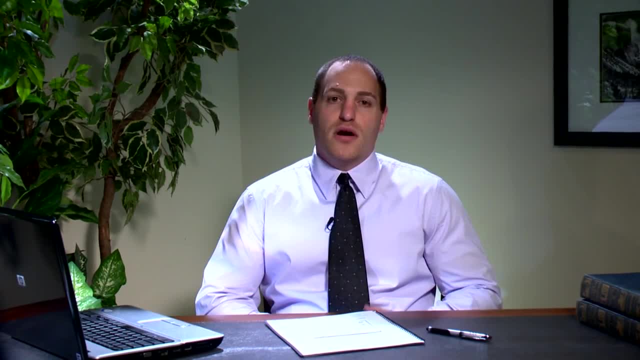 they're providing you with good value for money. Are these trademark attorneys giving you the time, attention and advice you need to make informed decisions? Are they going to go the extra mile for you? if an issue arises during the trademark registration process, Will they be available to? 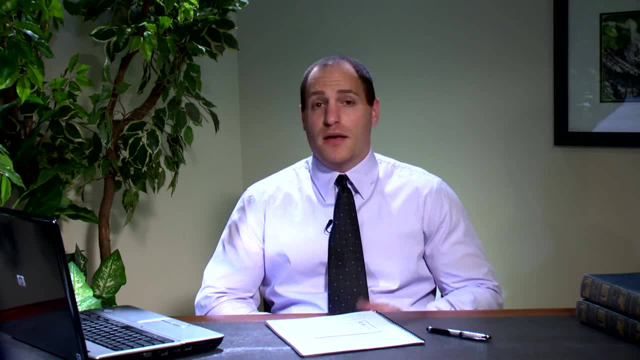 you to answer your questions and to address your concerns. Oftentimes, the answer is no, because, like most things in life, you get what you pay for. My goal is to provide you with professional, personalized and superior service at a reasonable price Every day.